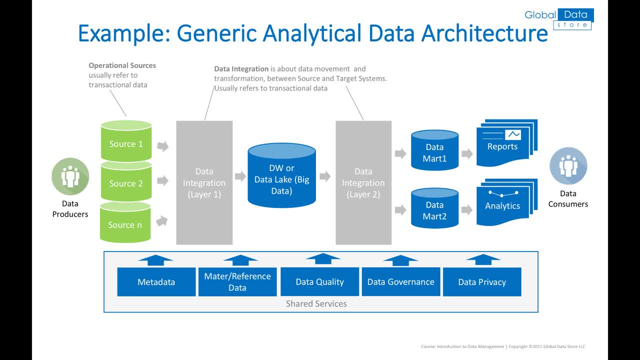 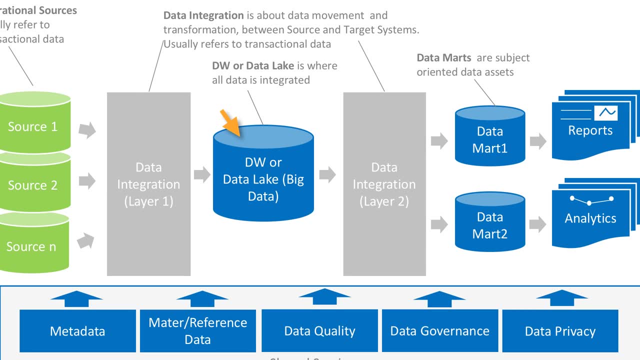 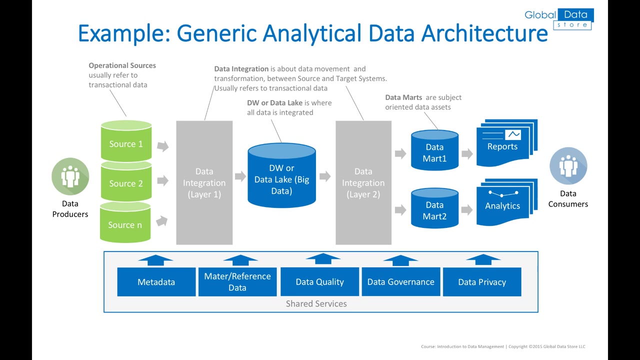 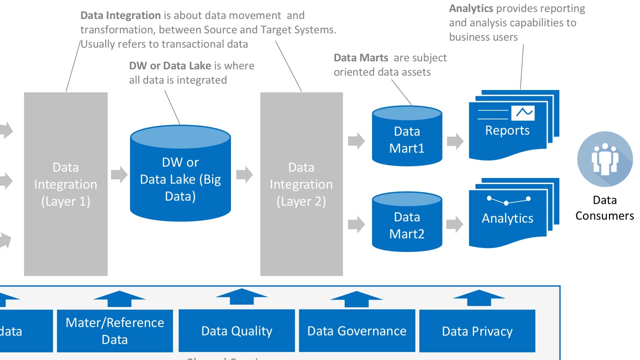 In addition, there are two static components. Data Warehouse or Data Lake refers to central data storage component where all data is integrated. On the other hand, Data Marks are subject-oriented data assets, that is, feed, Data Warehouse or Data Lake. Finally, there is Analytics Layer, which provides reporting and analysis capabilities to business users. 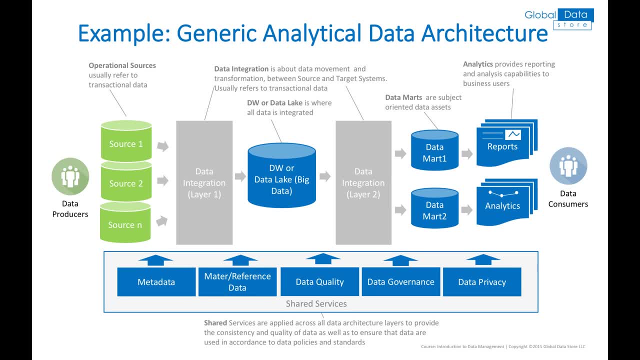 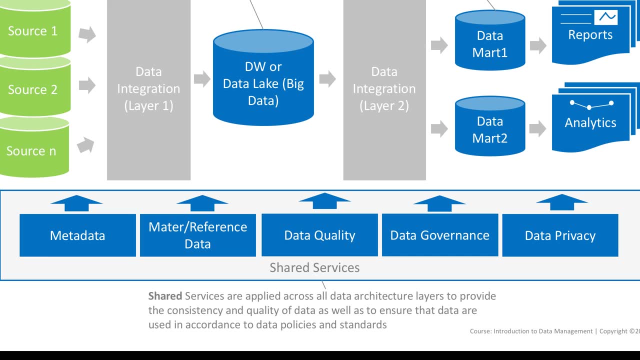 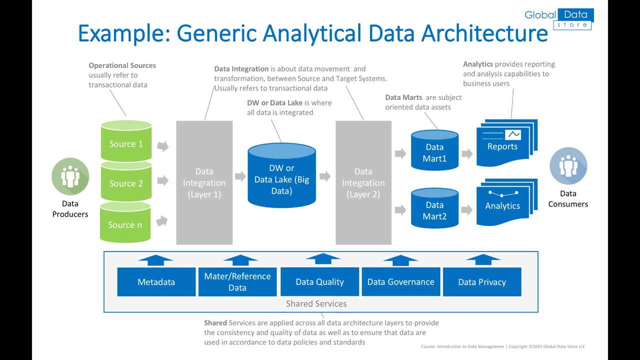 Last but not least, effectiveness and consistency of the data architecture is ensured by shared data services. Shared services are applied across all data architecture layers to provide consistency and quality of data, as well as to ensure that data are used in accordance to data policies and standards. 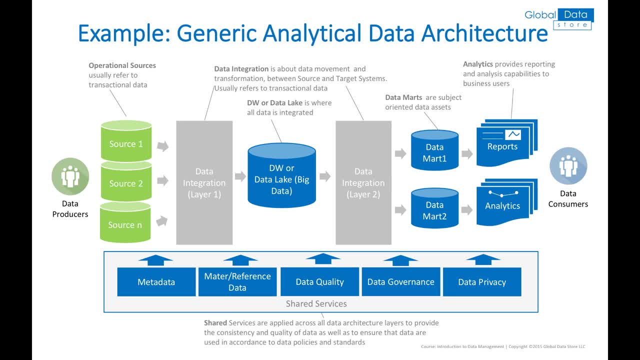 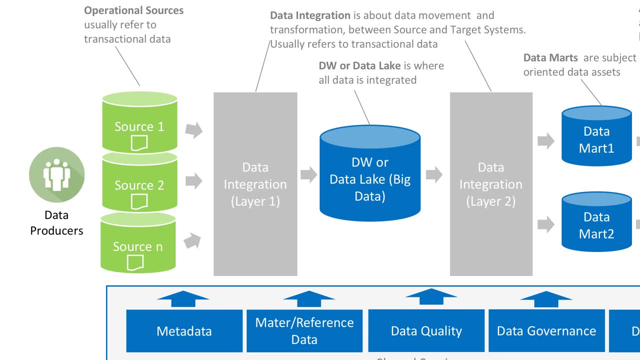 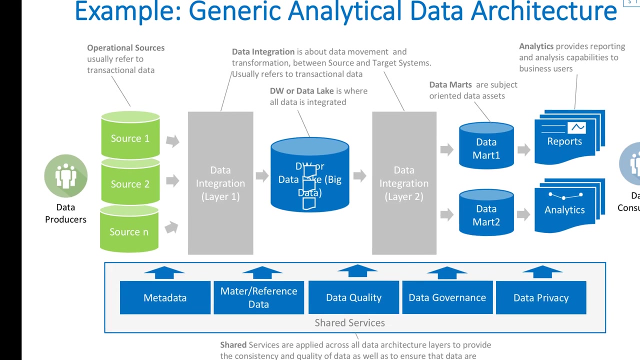 Let's see an animated example how data flows trough data architecture layers. In this example, we have selected DataPerfectLabsTVWeatherAети. It is used for edit andопасet materials such as Warm-up, Closton Potatoes, Quest or and spinning techniques. 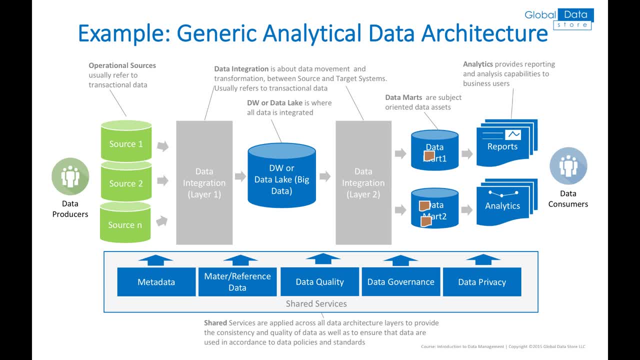 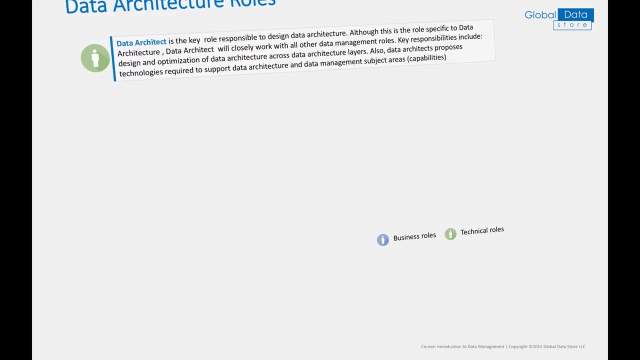 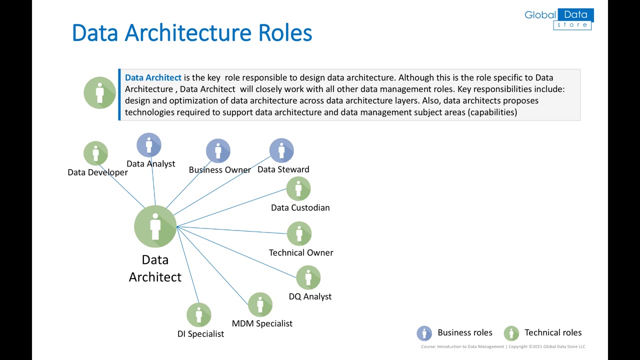 Data Warehouse was classed Senhorvaare. Data architect is the key role responsible to design data architecture. Although this role is specific to data architecture, data architect will closely work with all other data management roles. Key responsibility of this role includes design and optimization of data architecture across. 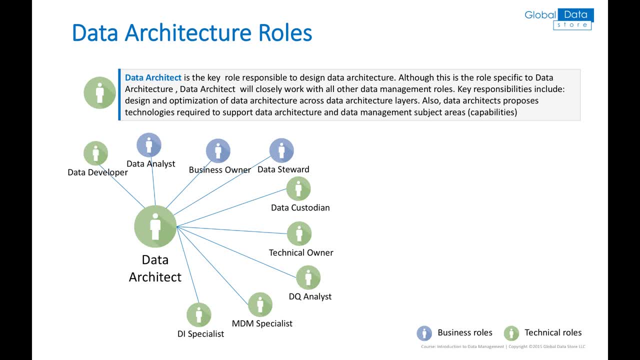 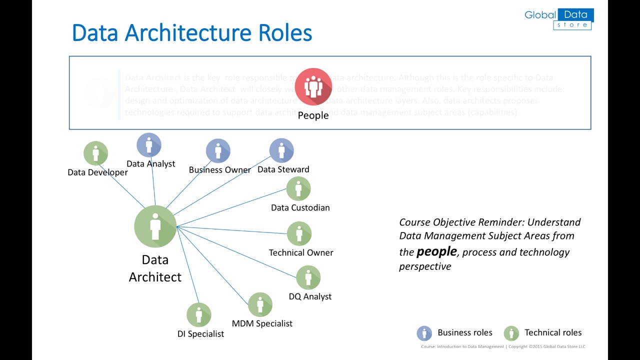 data architecture layers. Also, data architects propose technologies required to support data architecture and data management capabilities. In reference to course objectives: this slide covers people aspect of data architecture capability. In reference to course objectives: this slide covers people aspect of data architecture capability.